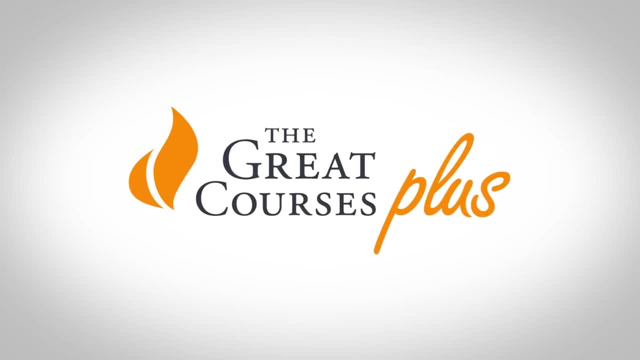 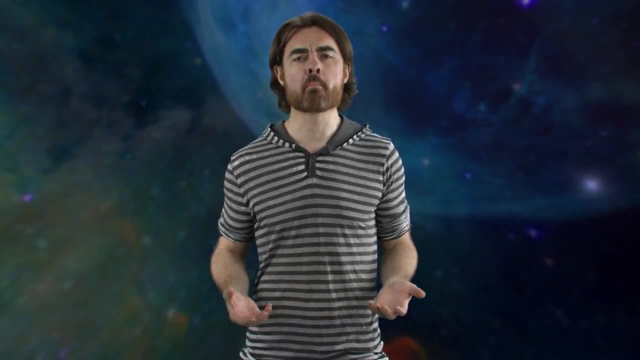 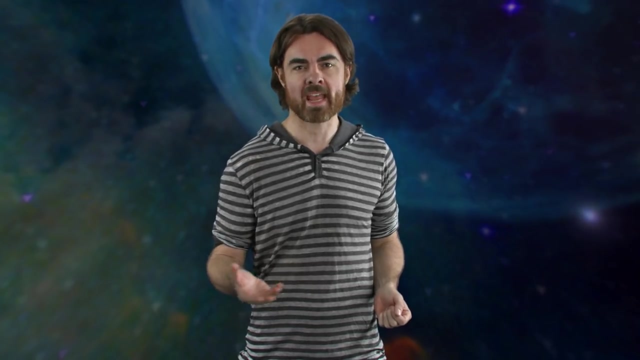 This episode is supported by The Great Courses Plus. The Planck constant defines the size scale at which the familiar physics of our macroscopic reality gives way to the weirdness of the quantum world. You might not expect the quantum behavior of the microscopic to be observable on all scales of the universe, but it is. 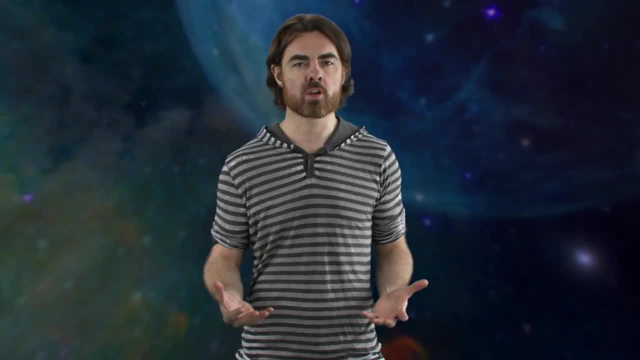 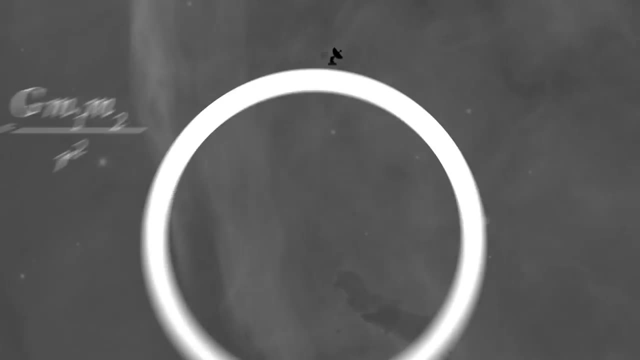 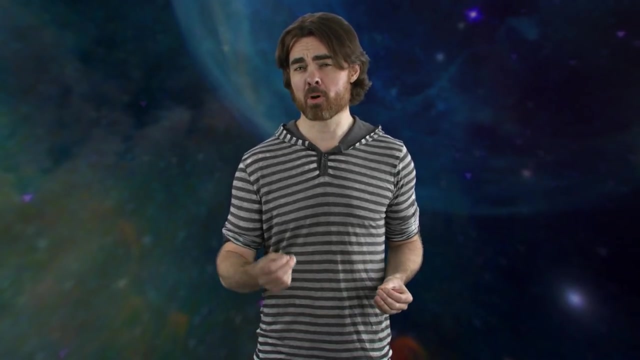 In fact, you can see the effect of this quantum behavior, and even measure the Planck constant, just by observing the color of sunlight. Zeno's famous paradox tells us that it's impossible to overtake a tortoise Run as fast as you like. 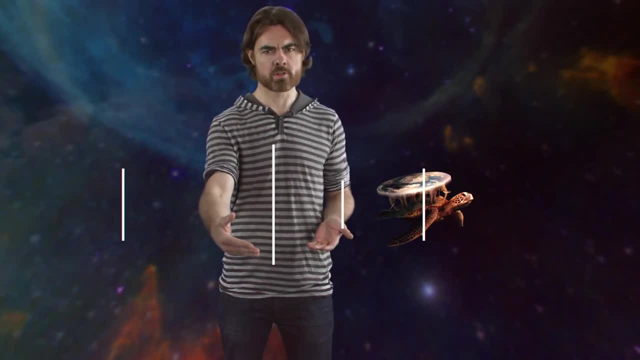 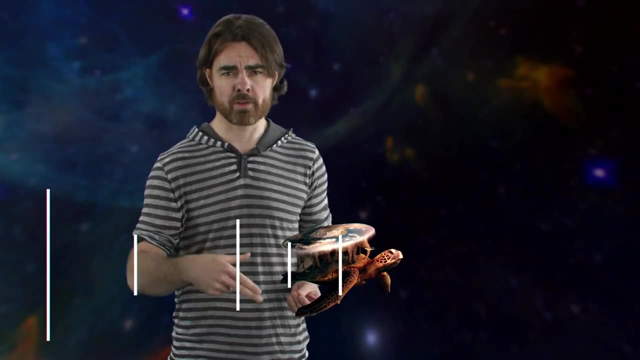 By the time you reach the tortoise's initial position, it'll have moved forward. Reach that second position, it'll have moved forward again. To overtake a tortoise, you need to travel to its previous position infinitely. That's infinite times. Each of those steps is shorter than the last, but there are still an infinite number of them. There are a few problems with this paradox, but one is that it assumes that space is infinitely divisible. This is not true, As your distance to the tortoise becomes unthinkably small. 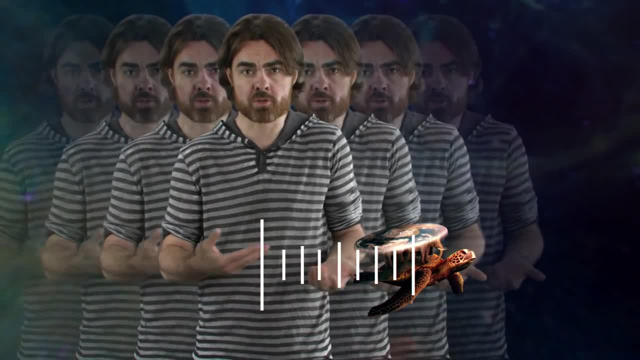 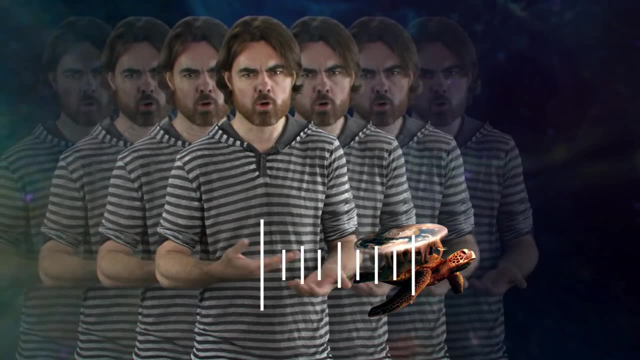 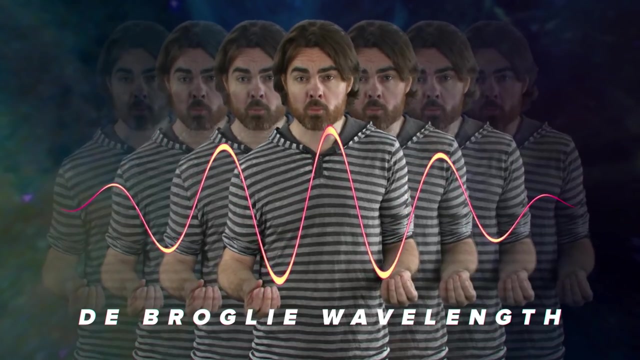 there arises a quantum uncertainty in your location, Get close enough to it, and this quantum blurriness means it's not possible to determine whether your location is really behind or in front of the tortoise. We talked about this recently when we discussed the de Broglie wavelength. 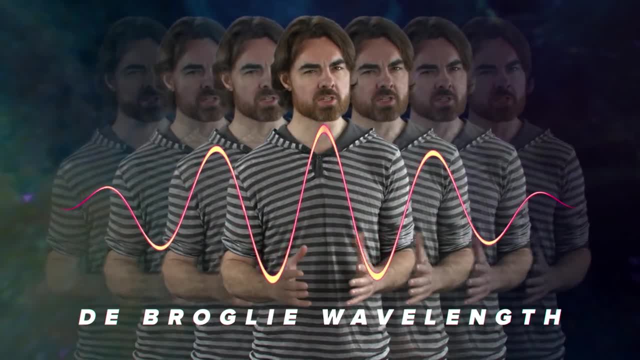 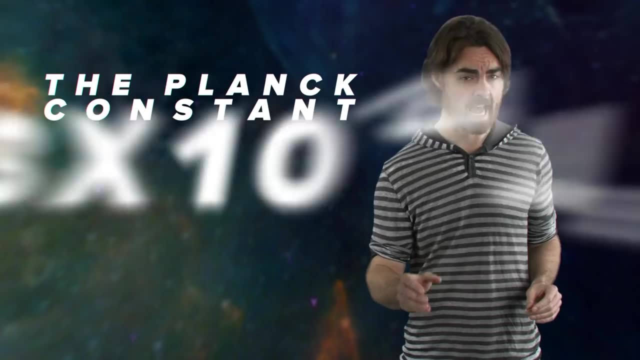 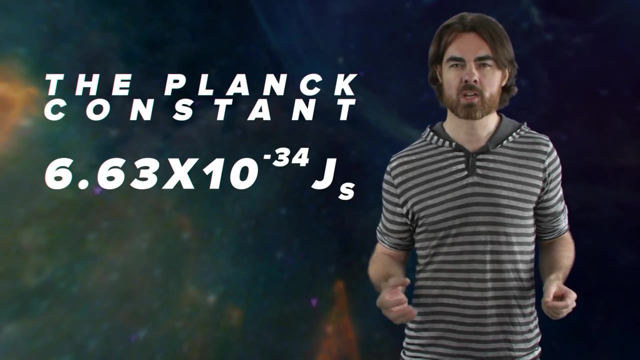 This, and more formally, the Heisenberg uncertainty principle, describes the smallest distance for which an object's location can be meaningfully defined. The tiny Planck, constant at 6.63 by 10 to the minus 34 Joules seconds, sets the scale of this quantum blurriness. 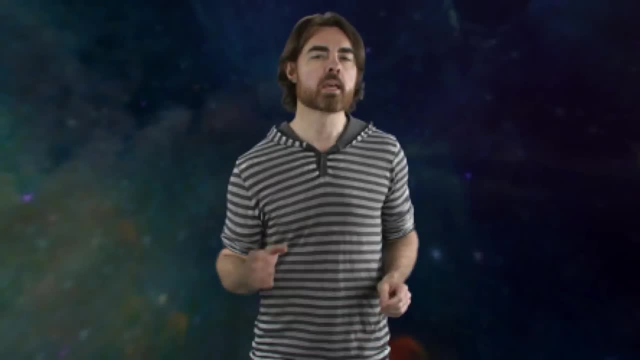 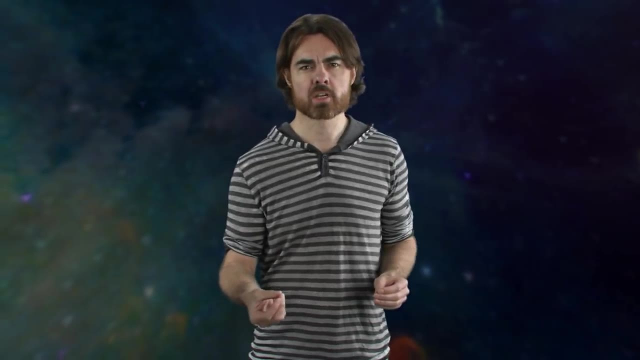 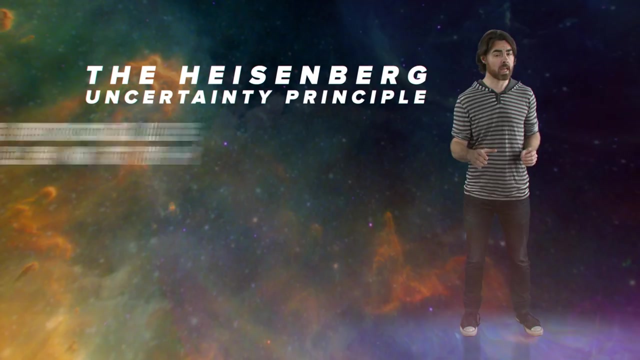 So it also sort of defines a pixelized pixel scale to reality. In many ways it defines the divisibility of the quantum world. In fact the Planck constant appears in essentially all equations that describe quantum phenomena, The Heisenberg uncertainty principle and the de Broglie. 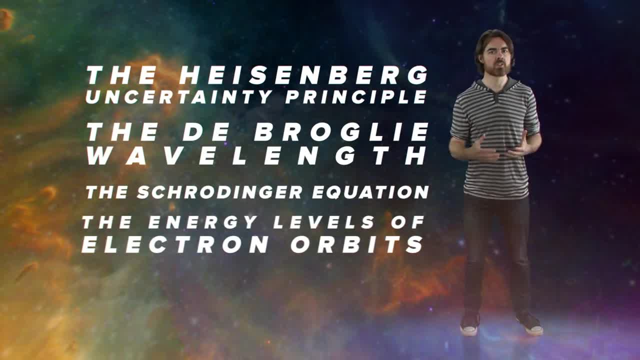 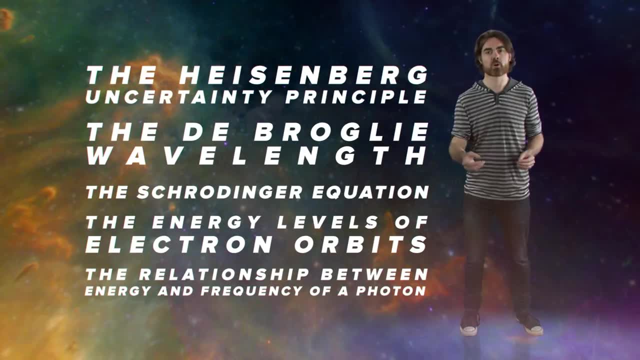 wavelength, but also the Schrodinger equation, the energy levels of electron orbits and, importantly, the relationship between the energy and frequency of a photon. It also sets the scale of the quantum world. It sets the size of the Planck length. 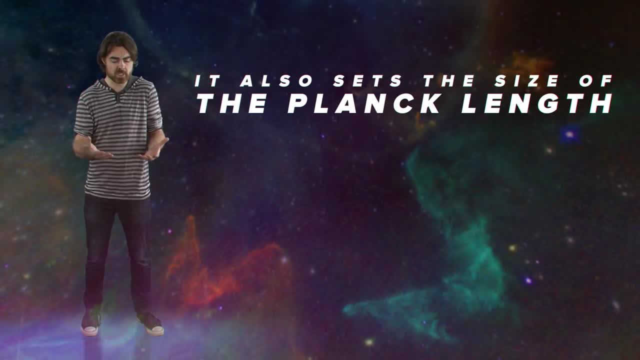 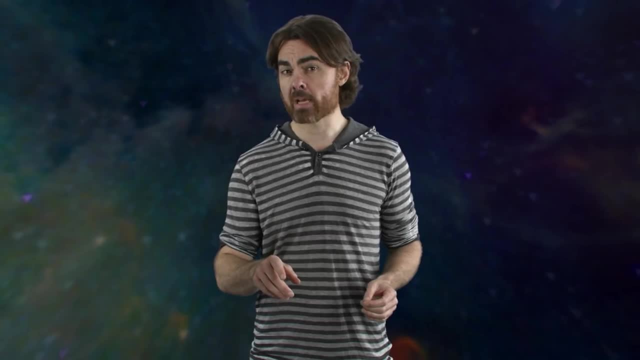 which is hypothetically the length below which the concept of length loses meaning. It may define the scale of quantum reality, but the influence of the Planck constant can be seen even on our scale, For example along with the sun's temperature. 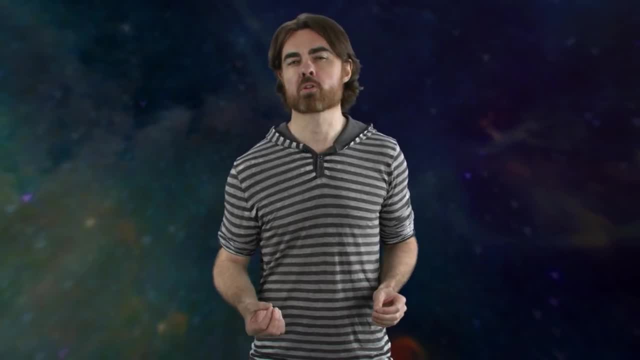 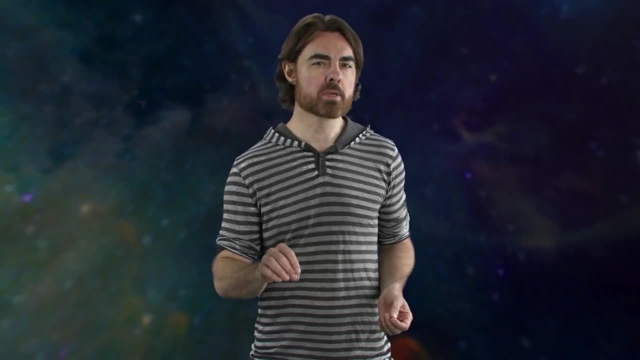 it sets the color of sunlight. If the Planck constant were 25% smaller, the sun would be violet, all else being equal. In fact, The mystery of why hot things glow the color that they do- led us to discover the quantum universe in the first place. 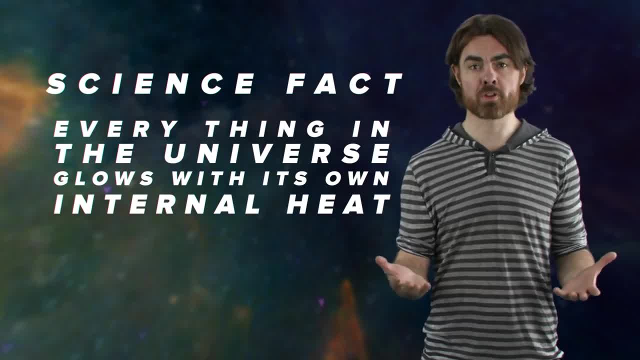 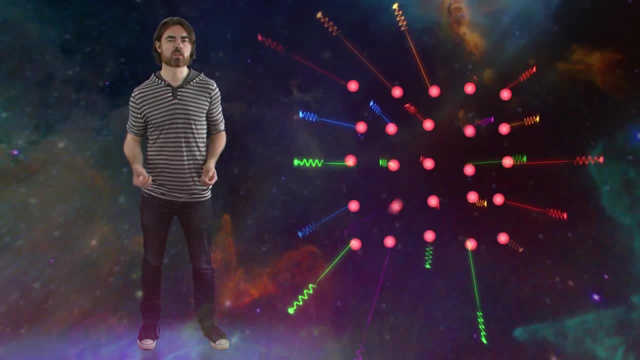 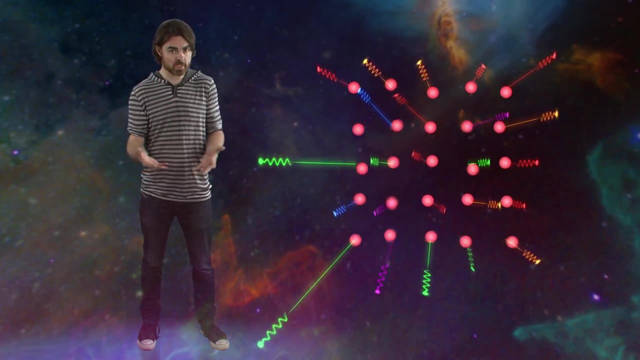 Science fact: Everything in the universe glows with the light of its own internal heat. Heat is just the energy in the random motion of particles comprising an object. Accelerated charges produce electromagnetic radiation light, and so an object made of jiggling charged particles. 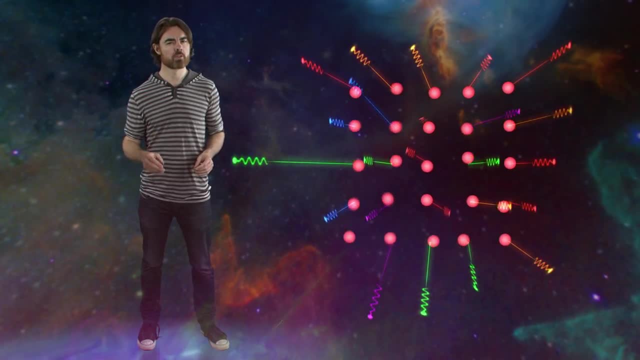 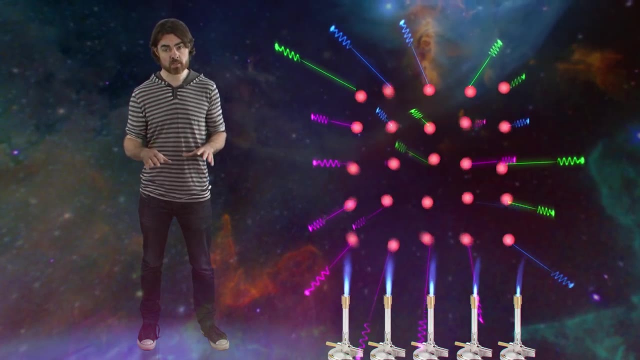 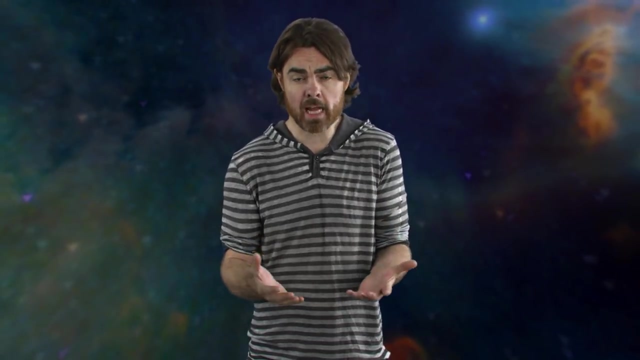 like electrons and protons, glows. The hotter an object is, the faster its particles jiggle, And so the average frequency of the resulting particles of light, of photons, increases with temperature. This average frequency defines the color that we see. 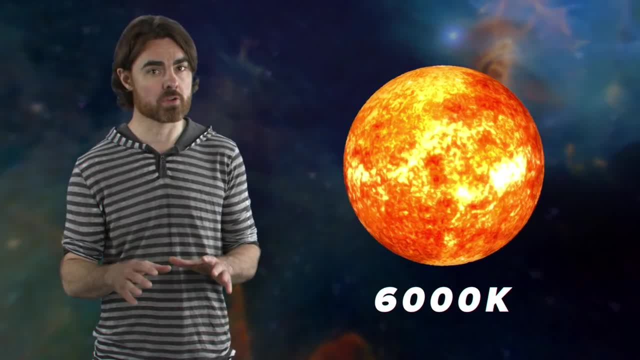 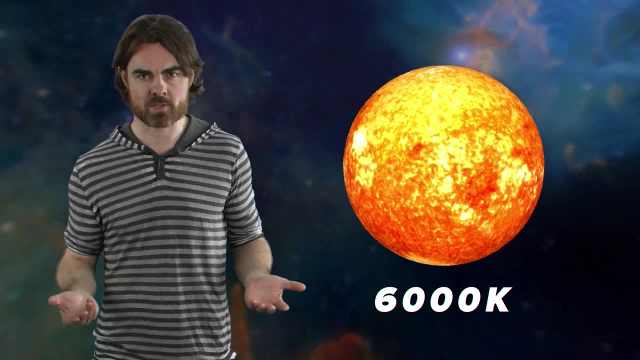 The sun is yellow because its 6,000 Kelvin surface produces more photons in the greeny yellow part of the electromagnetic spectrum than anywhere else. The blue supergiant star Rigel is 12,000 Kelvin, and so it pumps out. 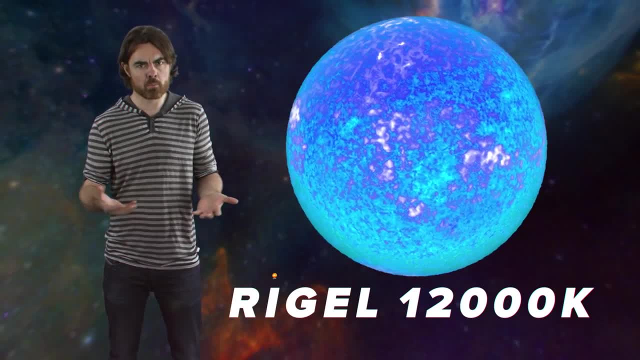 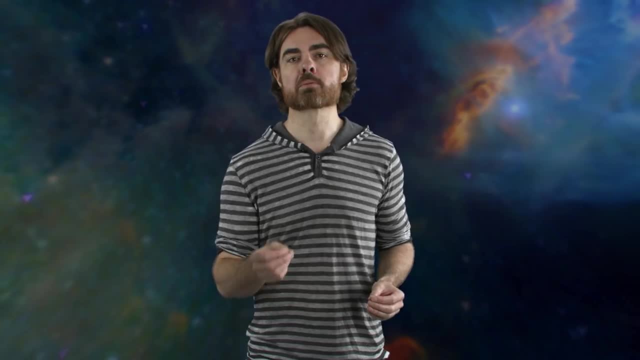 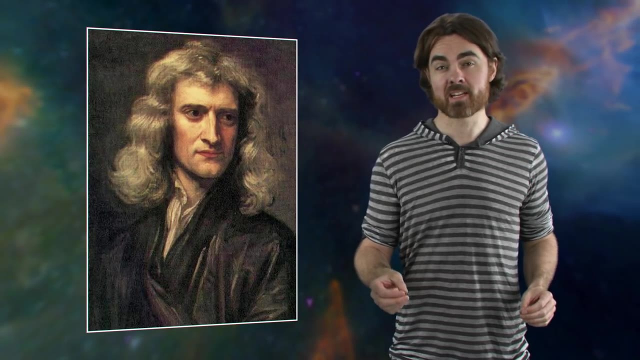 lots of high-frequency blue light and even more ultraviolets. Your temperature is around 310 Kelvin, so your heat glow is mostly in low-frequency infrared photons. It was Sir Isaac Newton who first analyzed this heat glow in the 1660s, when he used a prism to split sunlight. 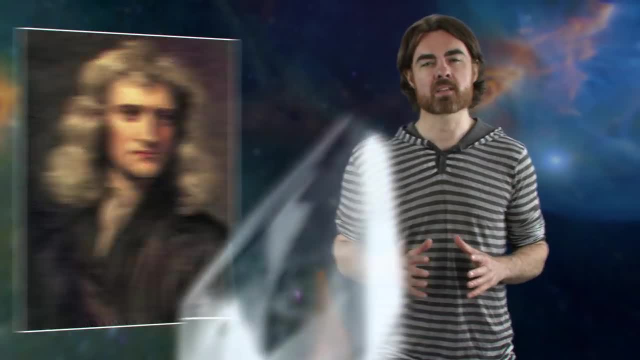 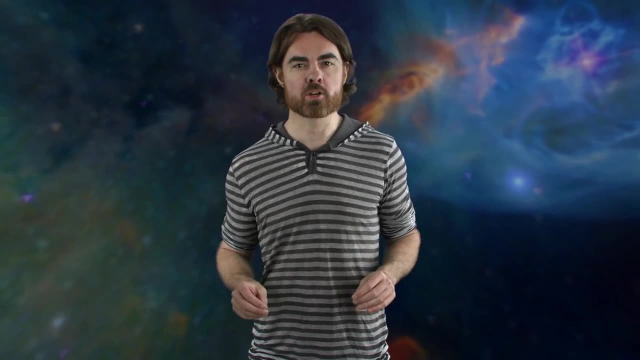 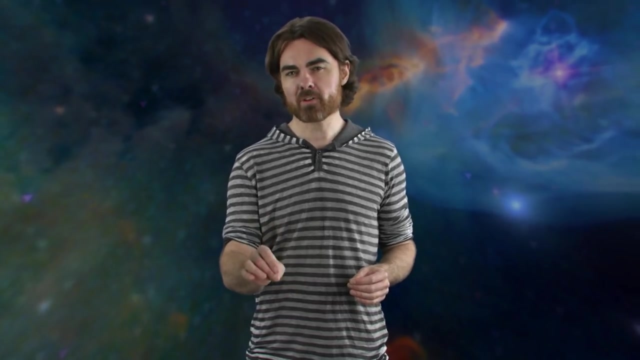 into its component colors, But he didn't realize that the relative brightnesses of those colors held the key to the quantum world. By the late 1800s the distribution of brightnesses with frequency produced by hot objects had been mapped in careful experiments that blacked out. 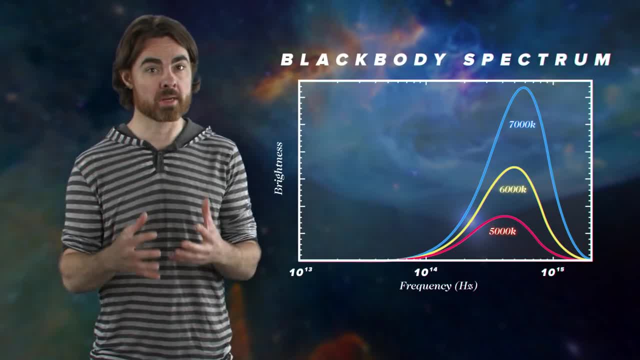 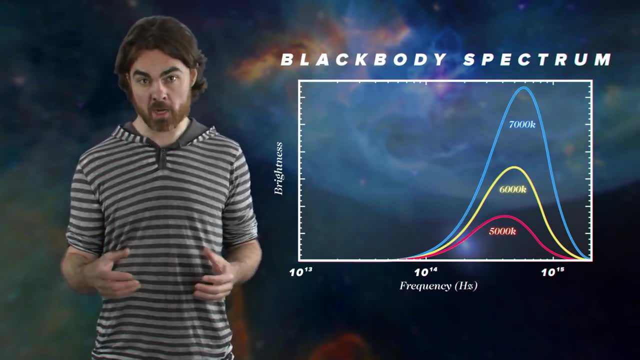 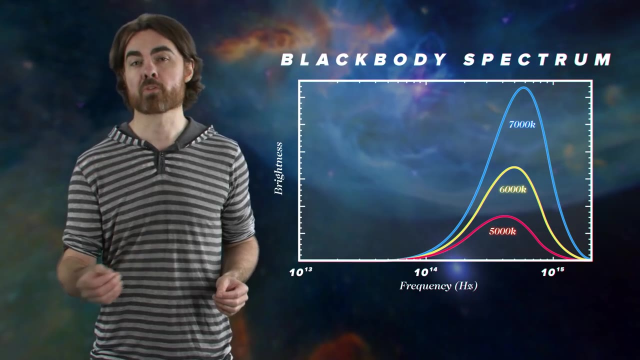 anything but the glow of heat. The resulting blackbody spectrum looks like a lopsided bell curve. However, the deep physics behind this shape remained a mystery. The key to unlocking the mystery lay in finding a mathematical description for the blackbody spectrum. 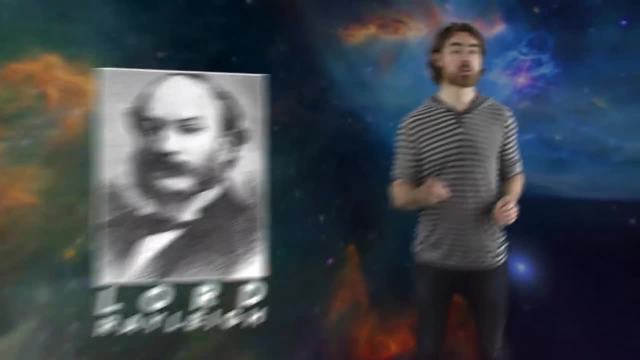 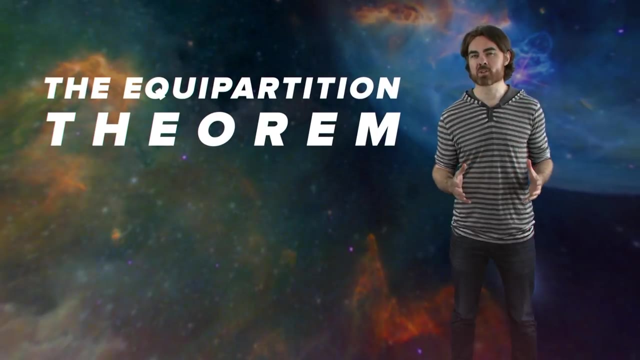 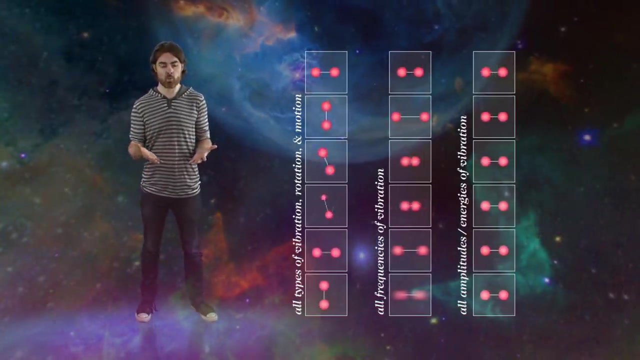 At the beginning of the 20th century a couple more Brits, Lord Rayleigh and Sir James Jeans, attacked the problem with a relatively new idea called the equipartition theorem. It states that an object's heat energy will end up jiggling all of its particles in all the ways. 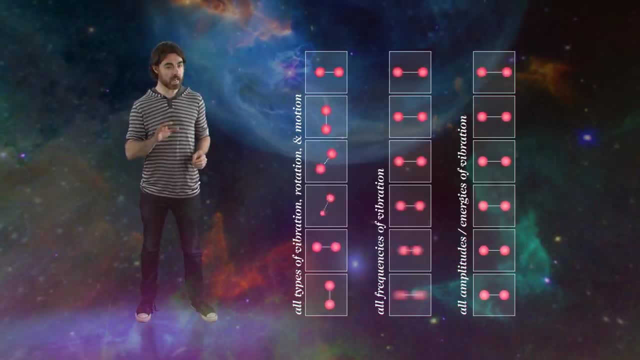 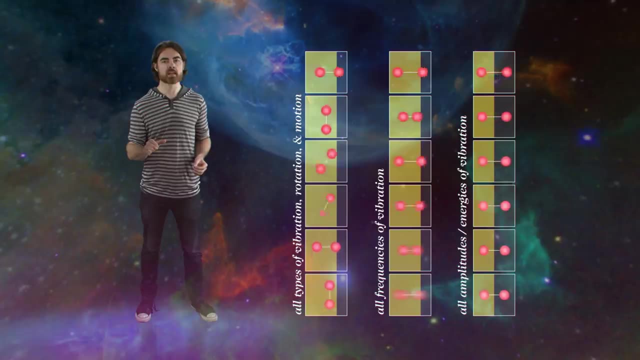 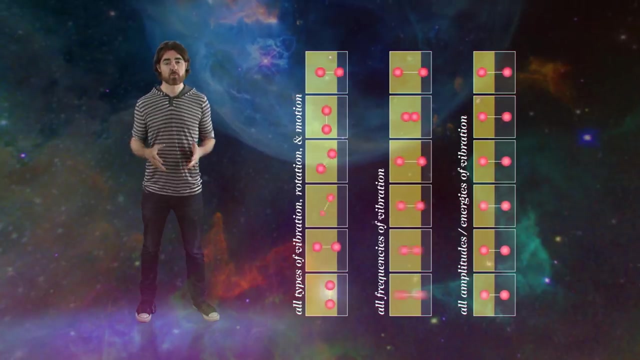 that they can be jiggled In. physics speak at equilibrium. energy is evenly spread between all possible energy states. This simple idea allowed our good Englishman to figure out the frequencies of the photons produced by all of this thermal motion. The resulting Rayleigh-Jeans law described the blackbody spectrum. 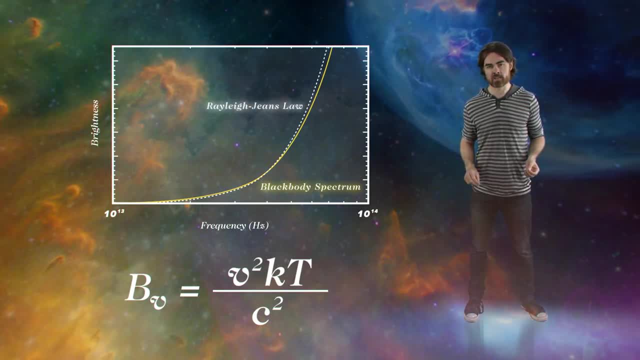 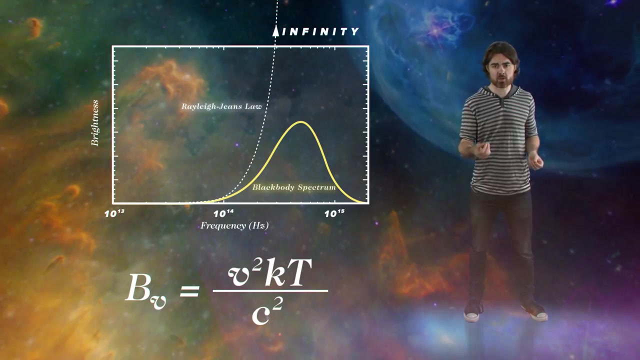 perfectly For low frequency infrared light, But for higher frequencies, like visible and ultraviolet, it predicted brightnesses that were way too high. Worse, it predicted that the intensity should eventually approach infinity, as frequency increased. It paints the crazy picture of a universe. 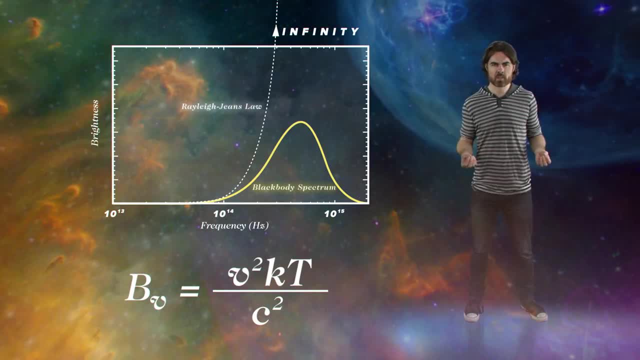 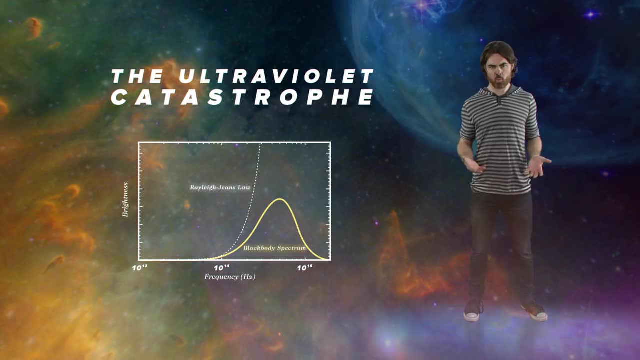 full of infinite extreme energy- gamma radiation. This appears not to be the case. This was called the ultraviolet catastrophe. It was catastrophic because it meant that something was fundamentally wrong with the classical physics that went into the Rayleigh-Jeans law. The problem turned out to be that in classical physics, 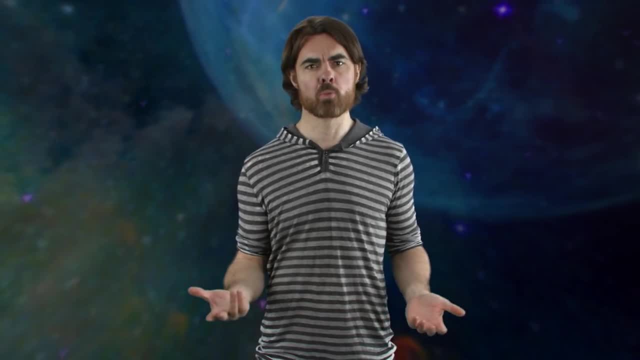 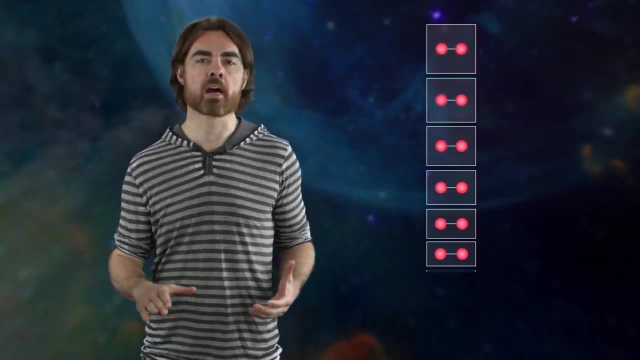 everything can be infinitely divided. infinitely divided, There's no smallest anything. The Rayleigh-Jeans calculation allows particles to vibrate with any amount of energy, all the way down to infinitesimally tiny wiggles. When they tried to mathematically distribute. 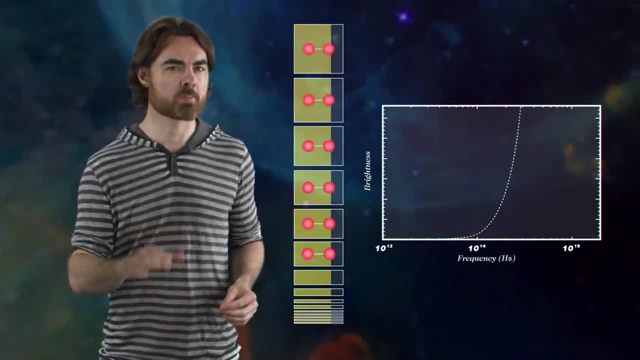 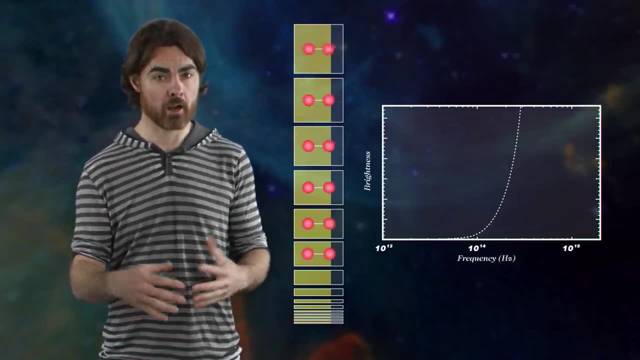 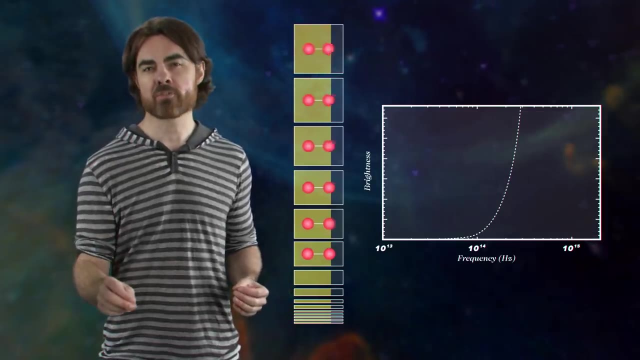 heat energy to equipartition it across possible energy states. way too much energy got packed into the countless very tiny energy states at high frequencies. Mathematically, Rayleigh and Jeans were chasing Zeno's tortoise, infinitely dividing the smallest remaining energy states. 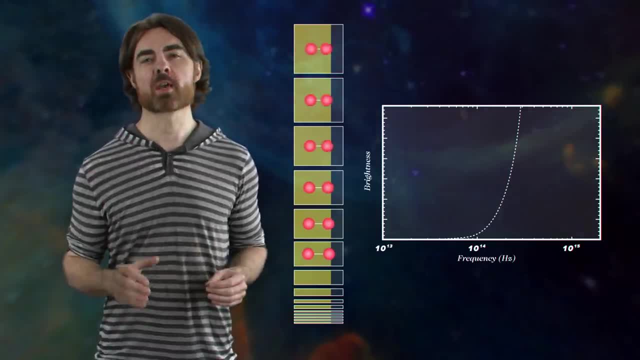 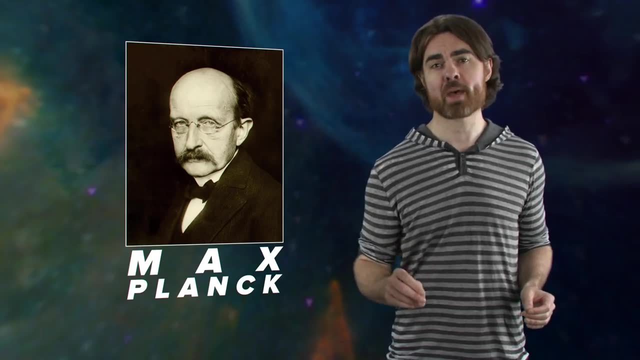 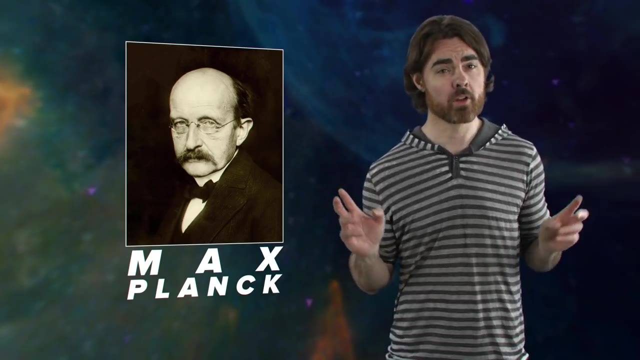 and so never ever finding an end to them. German physicist Max Karl Ernst Ludwig Planck resolved the catastrophe almost by accident, While searching for a new mathematical approach to deriving the blackbody spectrum. he needed some sort of math trick to count those supposedly. 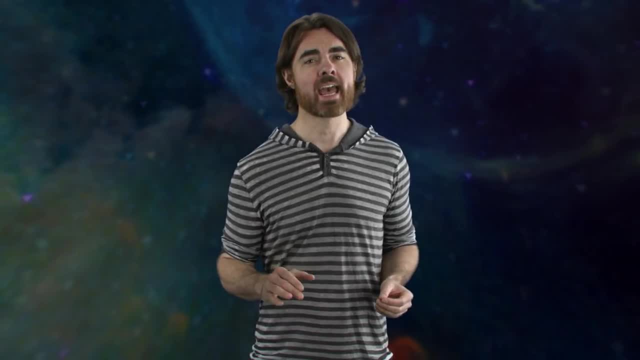 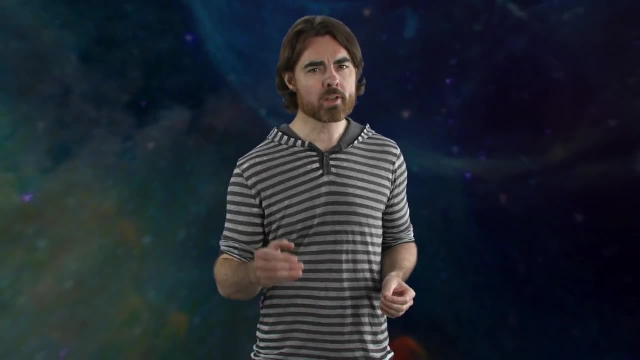 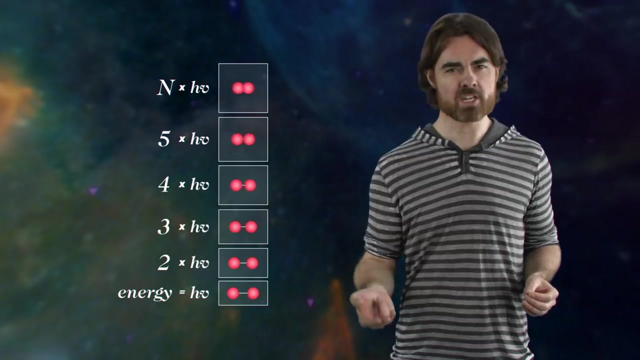 infinite energy states. In what he described as a moment of desperation, he tried something pretty silly. He decided that those particles could only vibrate with energies that were a multiple of some minimum energy. He quantized the energy states. He set this minimum energy to be the frequency. 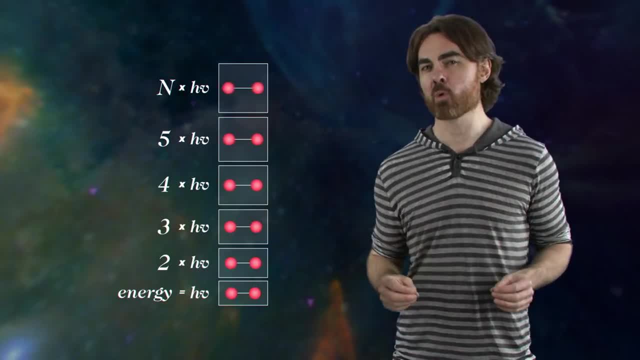 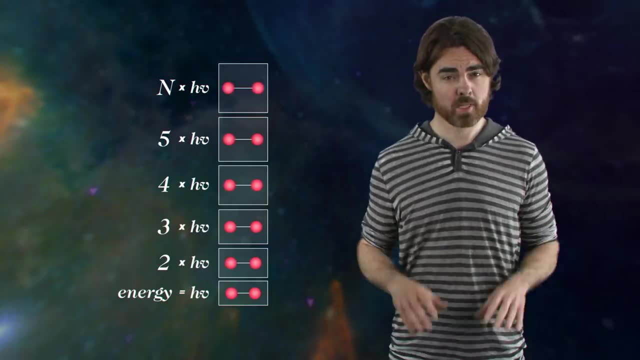 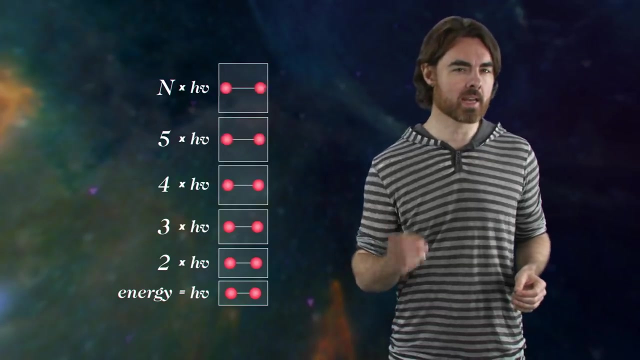 of a particle's vibration times, a very, very small number, a number that had yet to be measured. That number became the Planck constant. It was a move similar to smooshing your hands on the keyboard when your computer freezes, but it worked. 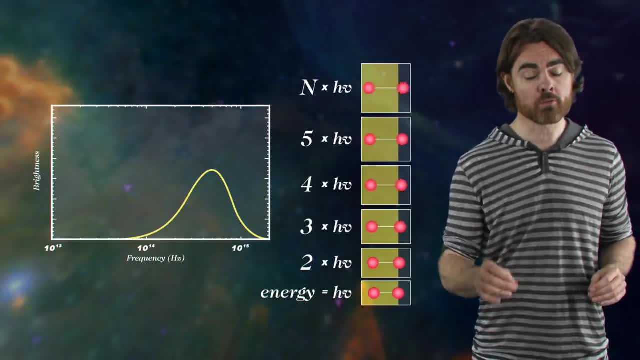 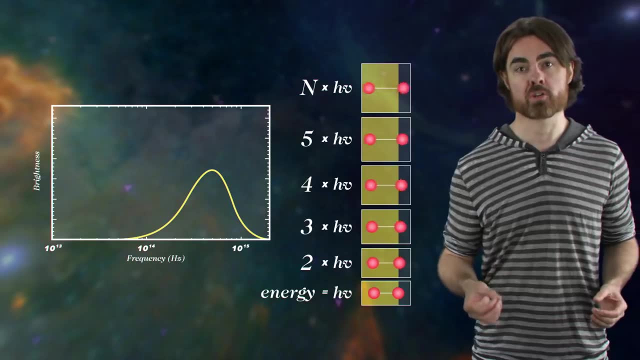 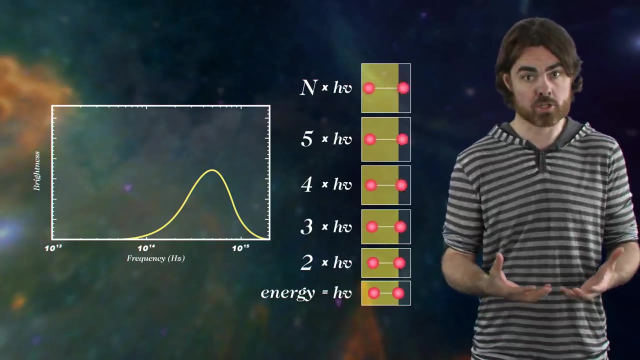 It allowed Planck to equipartition energy in a way that solved the ultraviolet catastrophe. Why? Because it limited how much energy those high-frequency vibrations could hold. Planck's new equation described the shape of the blackbody spectrum exactly across all frequencies. 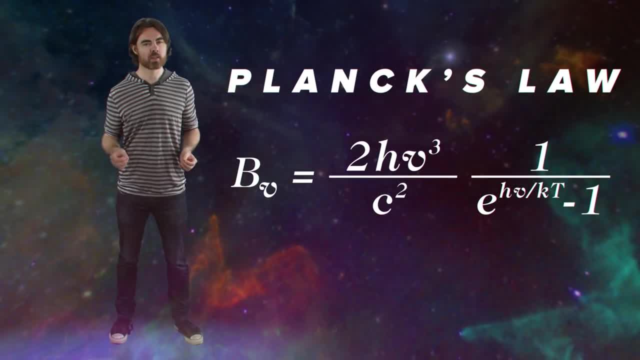 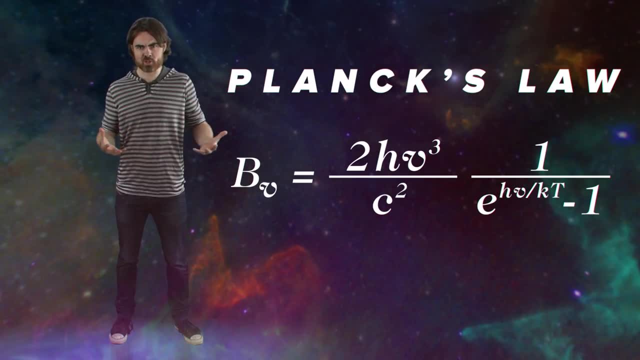 of light. It became Planck's law, Now Planck's. Planck didn't originally think that these quantized energy levels were real. It was supposed to be a math trick. He expected his new constant to turn out to be 0, which would mean no interval between energy states. 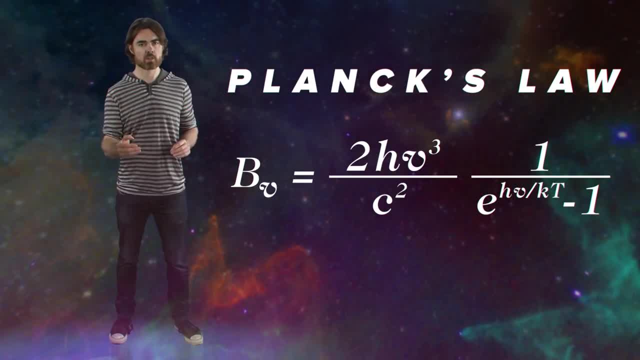 no quantization, no minimum energy. In that case the Planck constant would have canceled out in the final equation, but it didn't. The Planck constant is firmly entrenched in the Planck black body law. Energy quantization is real. 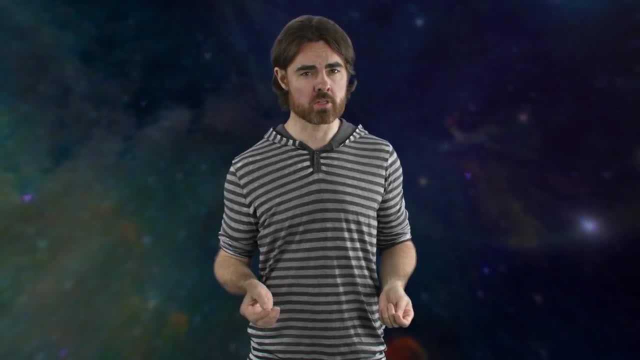 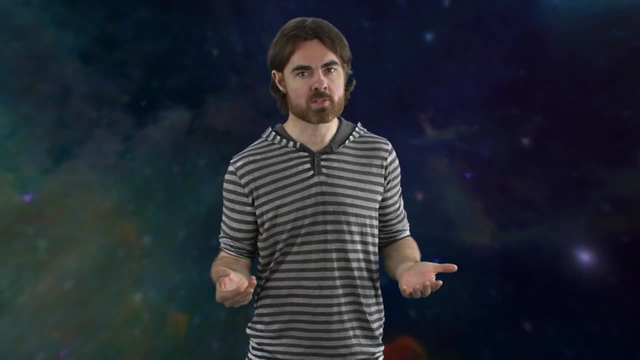 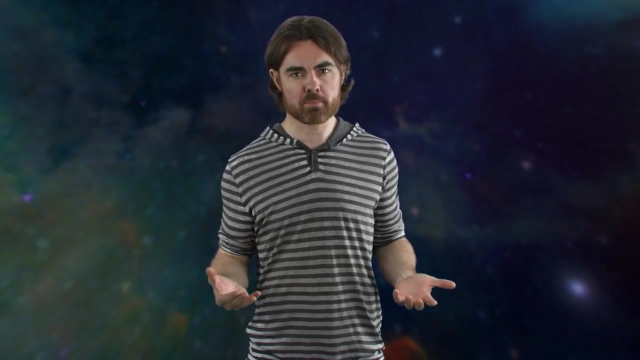 Now the actual value of the Planck constant still had to be measured. but given a mathematical form for the blackbody spectrum, it was possible to do this just by varying the constant until the Planck law matched the observed spectrum. But once you know the Planck law and an object's temperature, 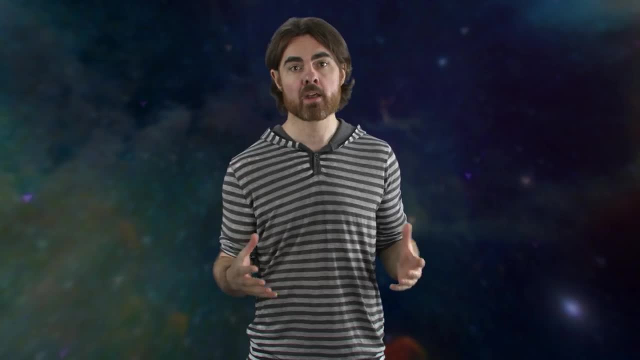 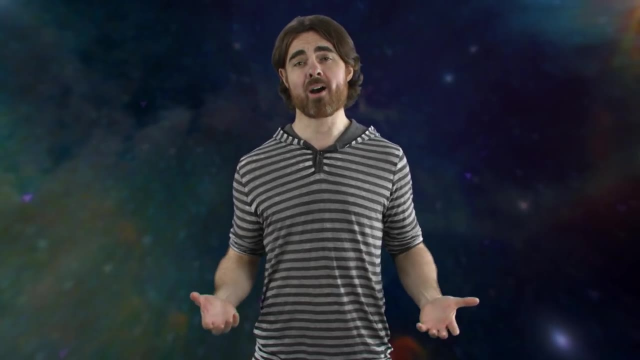 you can calculate the Planck constant just by finding the brightest part of an object's heat glow, For example by observing the color of the sun. As usual, it took Albert Einstein to fully understand the physics behind Planck's strange quantized vibrations. 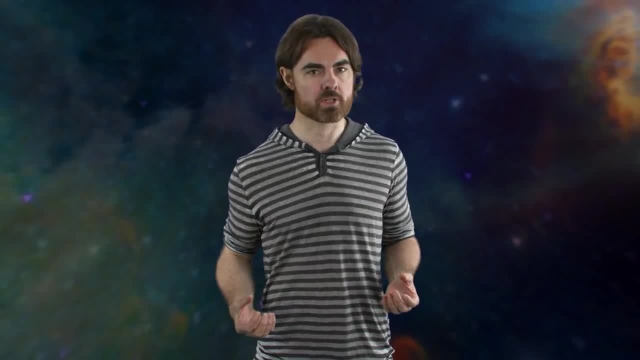 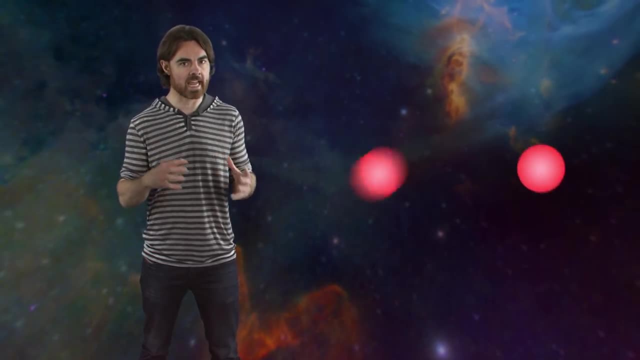 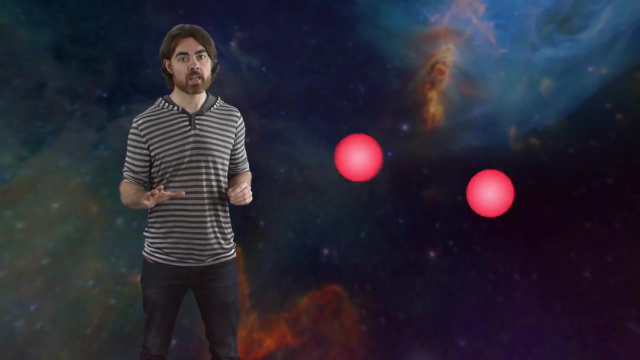 Einstein realized that it's actually light that is quantized. Those little vibrating particles do have quantized energies, but it's because they can only gain or lose energy by absorbing or emitting one particle of light at a time, And that light comes in indivisible energy. 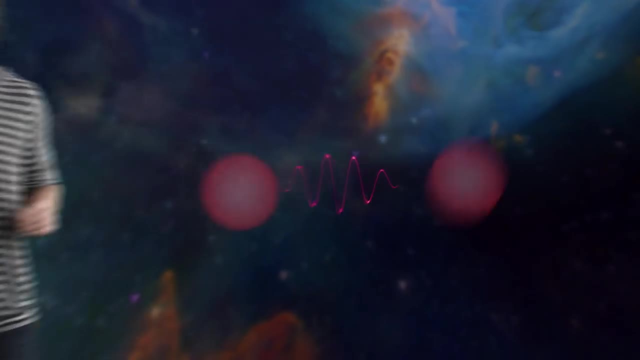 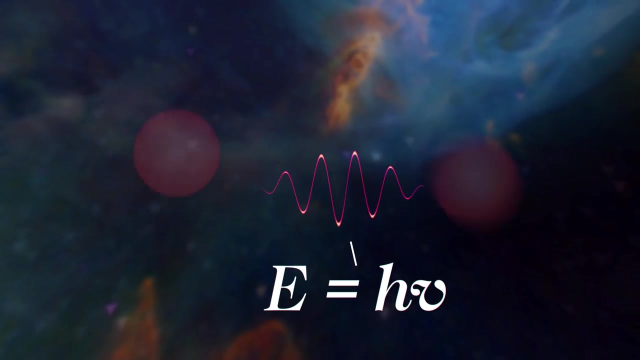 packets. Planck's discovery was the clue Einstein needed to hypothesize the existence of the photon part wave part particle carrying a quantum of energy equal to the now familiar frequency of the wave times, the Planck constant. Einstein proved this through the photoelectric effect. 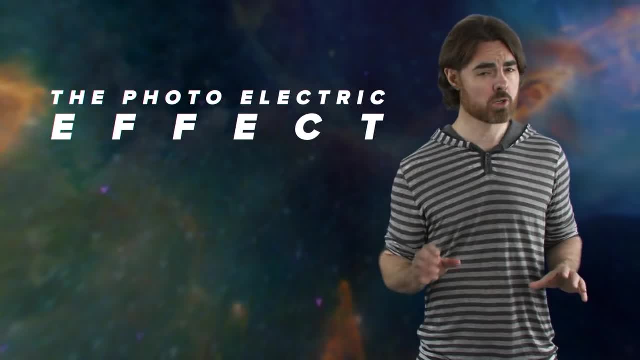 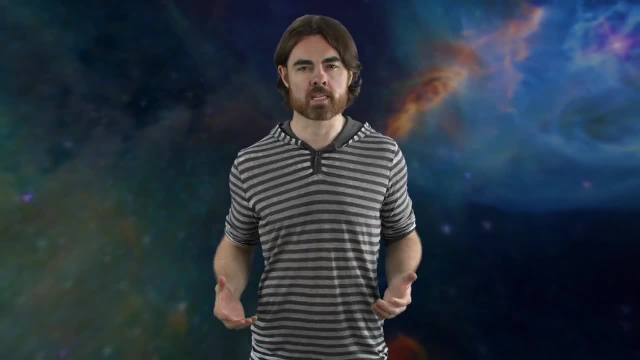 It got him the 1921 Nobel Prize in Physics, shortly following Planck's Nobel of 1918. These discoveries sparked a frenzy of sciencing that led to the quantum revolution of the 1920s And that little number that Max Planck came up with in his moment. 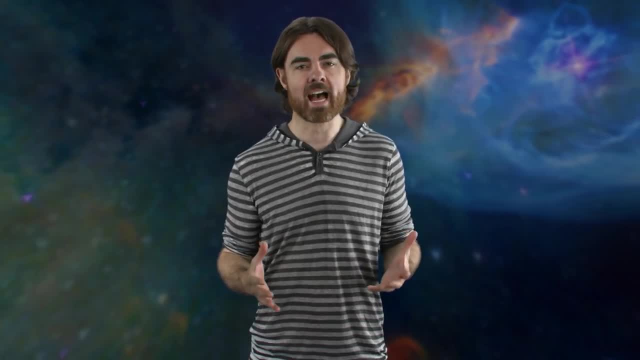 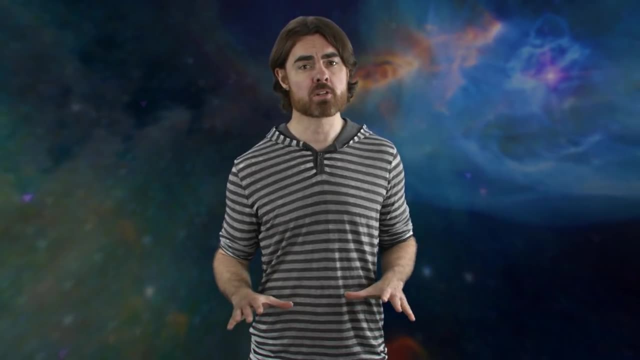 of desperation. the Planck constant remains at the heart of all things, quantum, But not just quantum. By defining the shape of the blackbody spectrum, the Planck constant can be read in the color of the sun and the stars, in the brightness of the different colors. 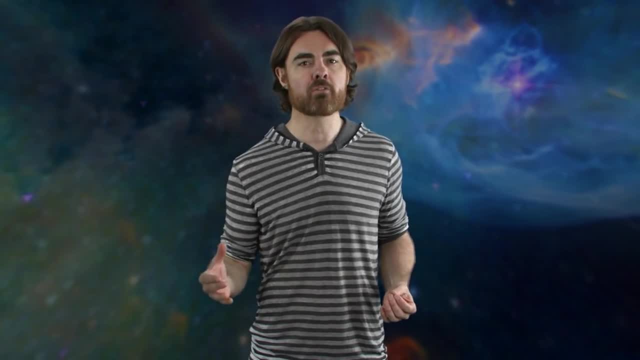 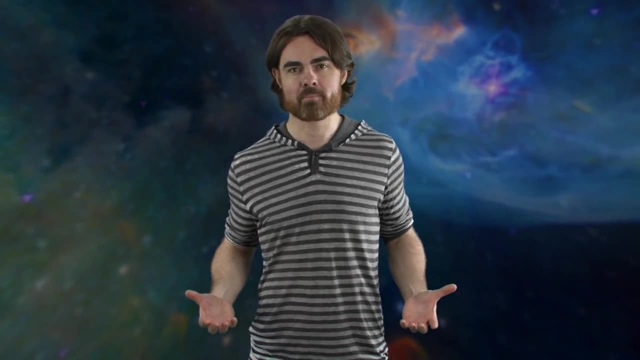 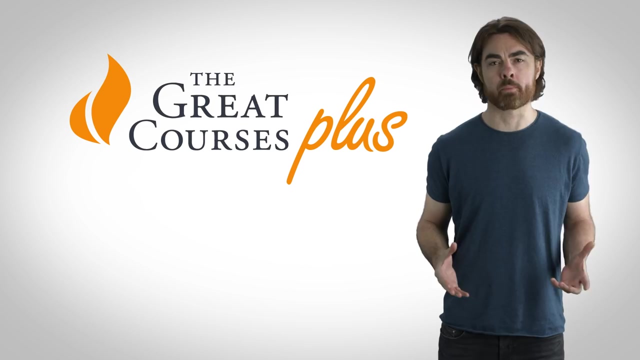 of the rainbow and, combined with a small handful of other fundamental constants, it governs the behavior of everything in this spacetime. Thanks to The Great Courses Plus for sponsoring this episode. The Great Courses Plus is a service that allows you to learn about a range of topics. 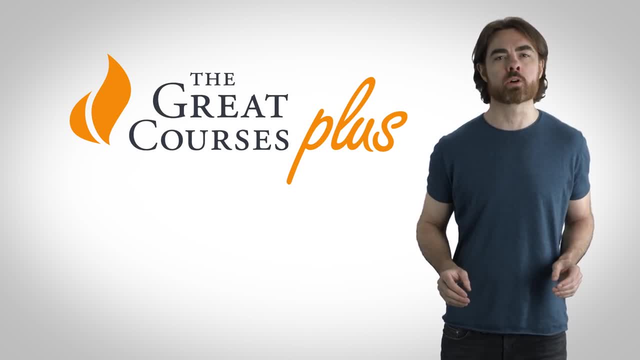 from Ivy League professors and educators from other schools around the world. Go to thegreatcoursespluscom. slash spacetime and get access to a library of different video lectures about science, math, history, literature or even how to cook, play chess, become a photographer, new subjects. 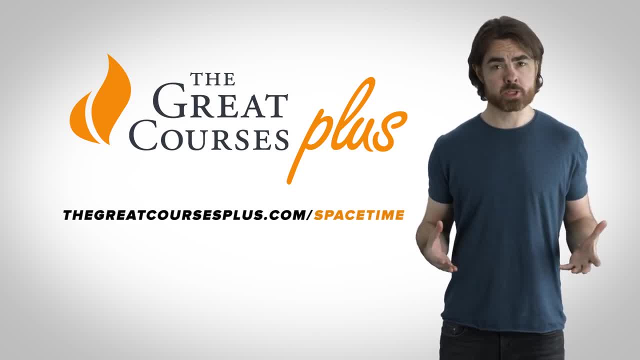 lectures and professors are added every month. With The Great Courses Plus, you can watch as many different lectures as you want, anytime, anywhere, without any tests or exams. Help support spacetime and start your one-month trial by going to thegreatcoursespluscom slash spacetime. 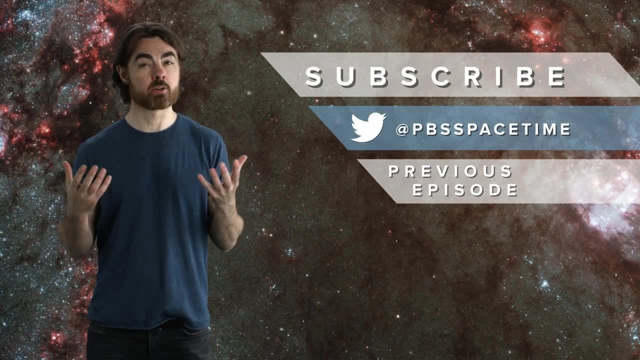 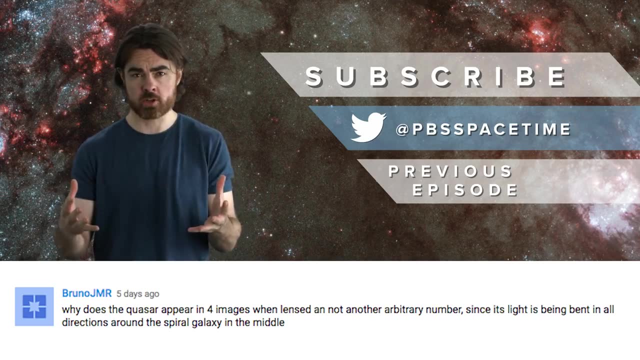 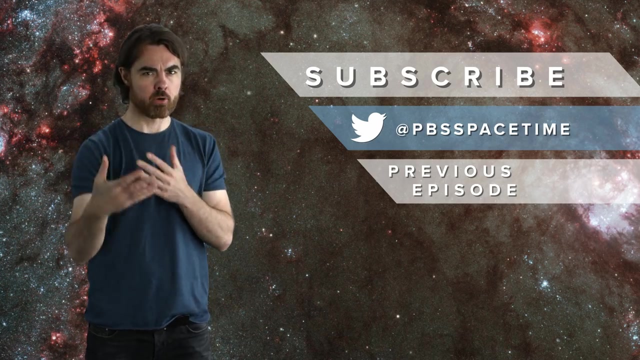 Last week we talked about gravitational lensing And you guys asked all the good questions. OK, a lot of you wanted to know why it is that the Einstein cross is a cross rather than a full ring. So if your light source, your lens and your telescope 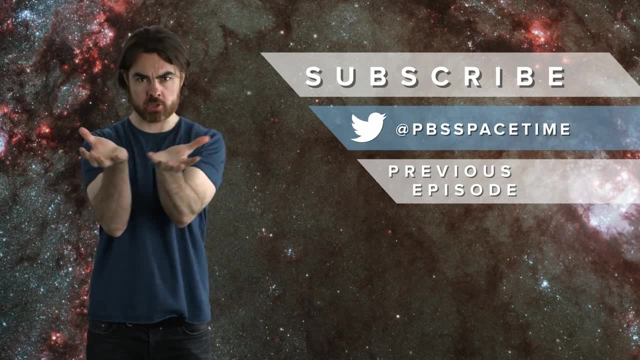 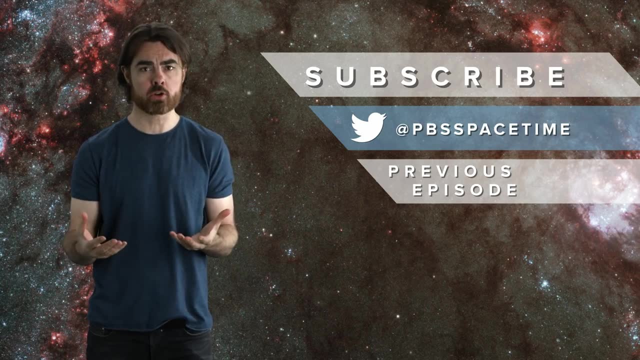 are all perfectly lined up and your lens is perfectly circular around the line connecting the three- the optical axis- then the light source will be stretched out into a circle. We call that an Einstein ring. In that case, all of the paths around the lens 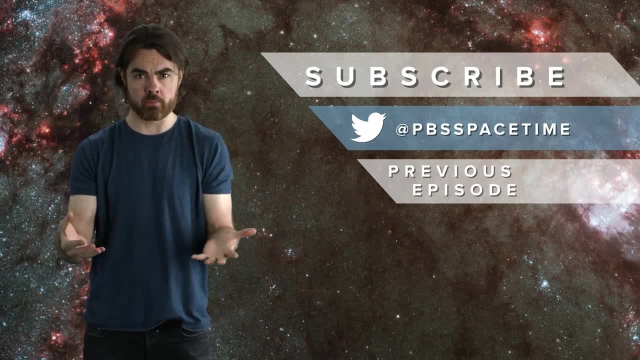 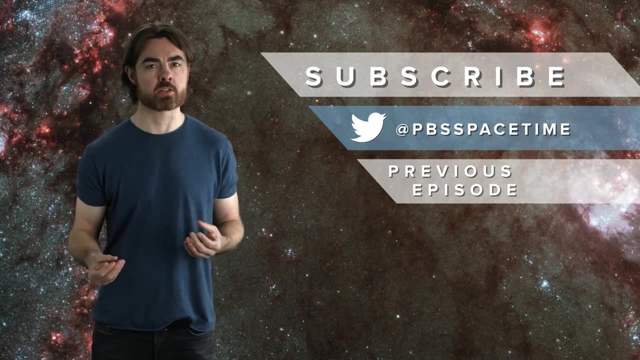 are equally good and so light from the source can travel all of them. But perfect alignment is almost impossible for something as small as a quasar. The quasar is always a circle. It's always slightly offset from the optical axis. Also, the lens' mass distribution. 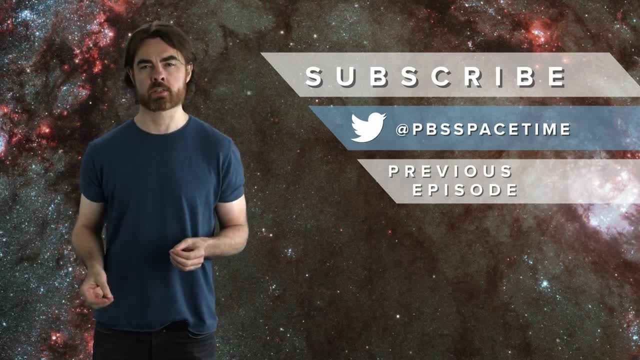 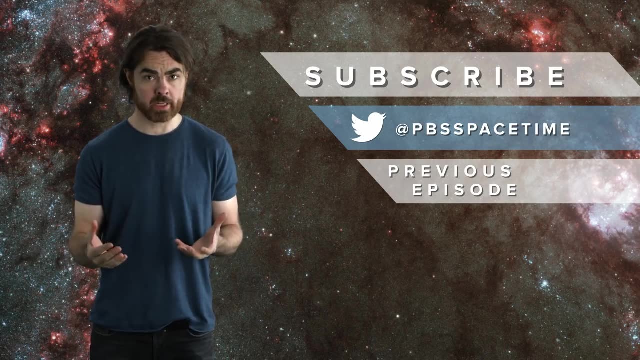 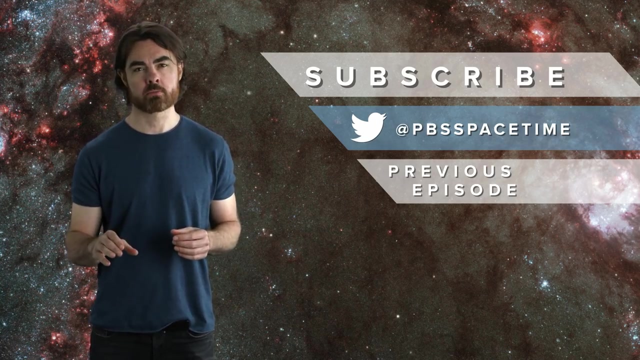 is never perfectly circularly symmetric around this axis. It's elongated in one direction or another. The result is that only a few paths around the lens get deflected directly back to us. If the alignment is still pretty close, then you see four images. 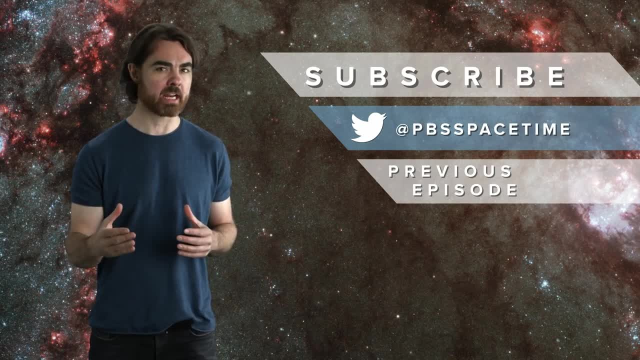 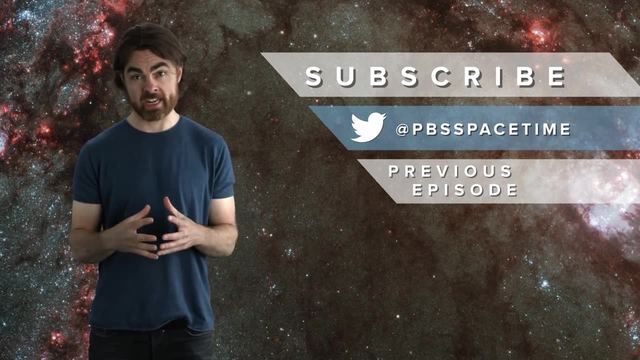 In fact there's really five: four magnified images and one heavily demagnified image in the center that we can't see. On the other hand, if the light source is large, for example an entire galaxy, then it's easier for at least part of the galaxy. 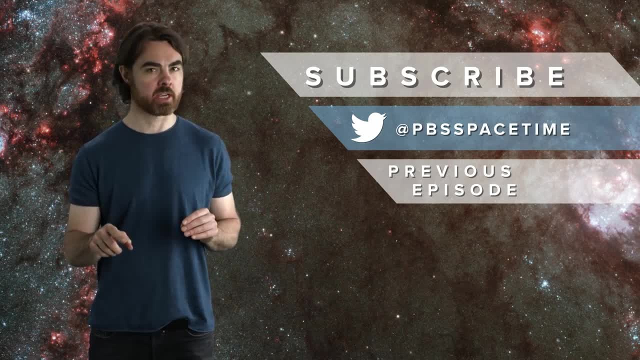 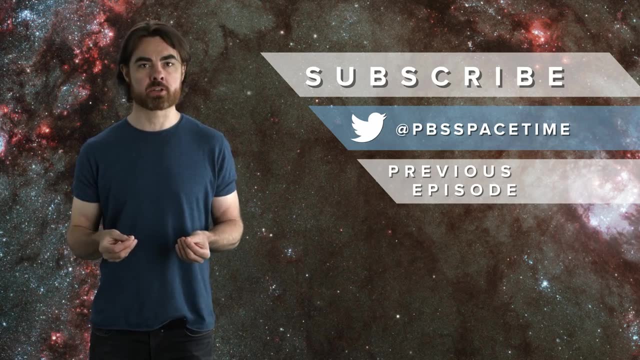 to be located directly on the optical axis. Then you'll see an Einstein ring. There are some cases where you see four individual quasar images connected by an Einstein ring. That Einstein ring is actually the galaxy that hosts the quasar. Gary Palmer would like to know how we can really 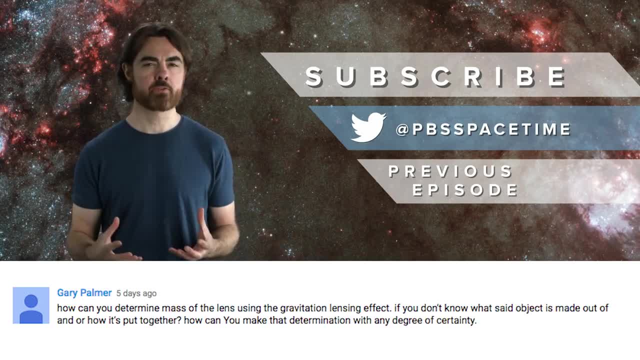 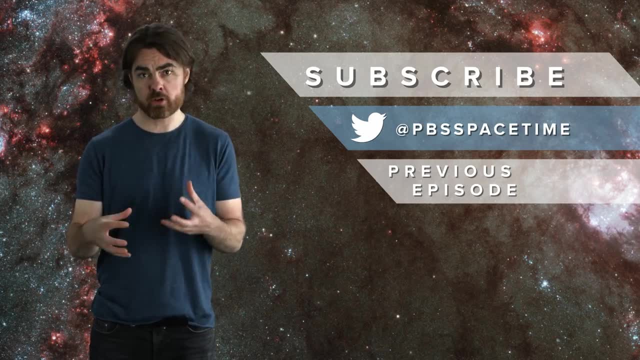 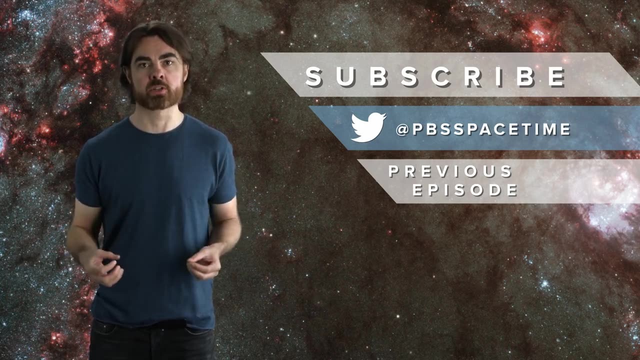 be confident measuring the mass of a gravitational lens, given we don't really know the composition of that lens. Well, it's true that for a given lens, there could be a range of different configurations of matter that produce the same distribution of light seen in the lens. so image positions and brightnesses. 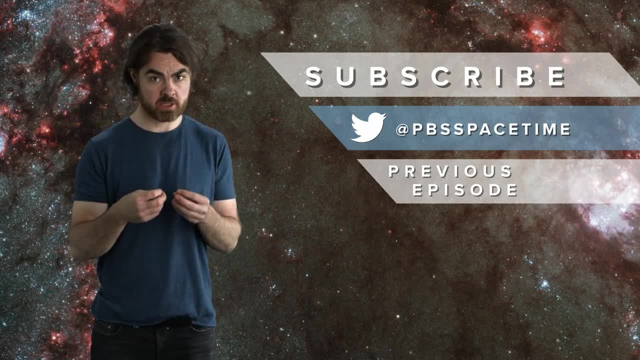 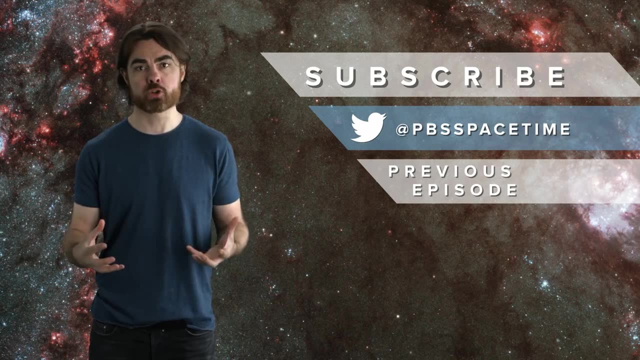 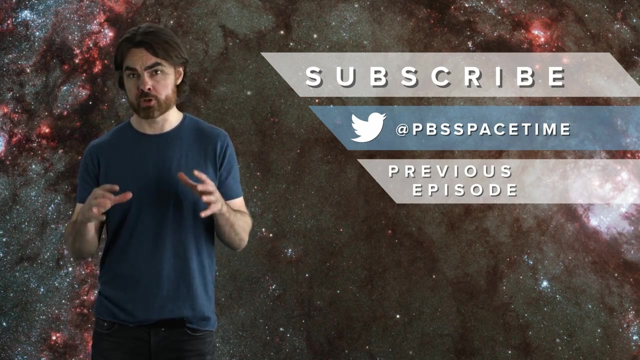 But if you know the distance to the light source and the distance to the lens, both from redshift, then you can explore an enormous range of possible lens mass distributions with computer simulations. So you end up with a set of virtual visual lenses that can reasonably 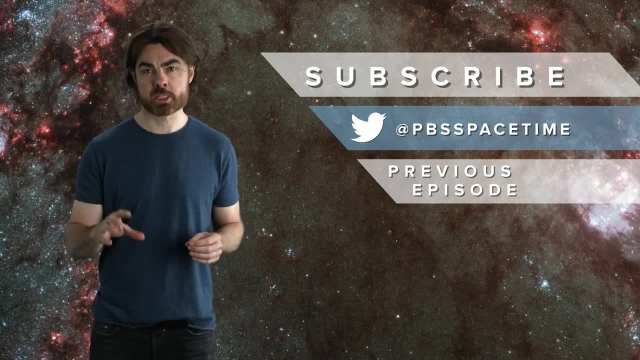 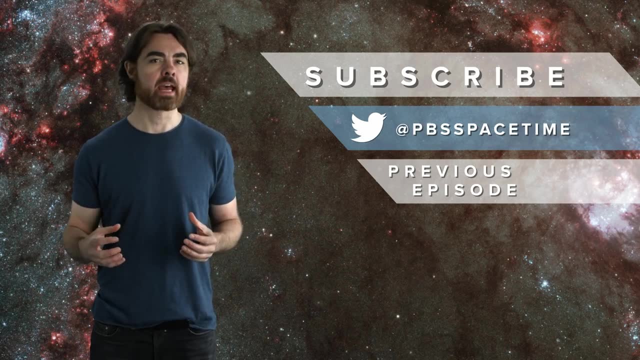 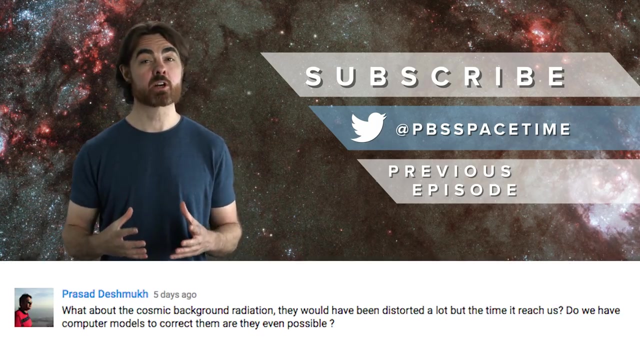 produce the observations. That set will span a range of masses, but that range is usually pretty small, So we end up with a best mass and error bars defined by that range. Prasad Deshmukh and a few others asked: is the cosmic microwave background radiation? 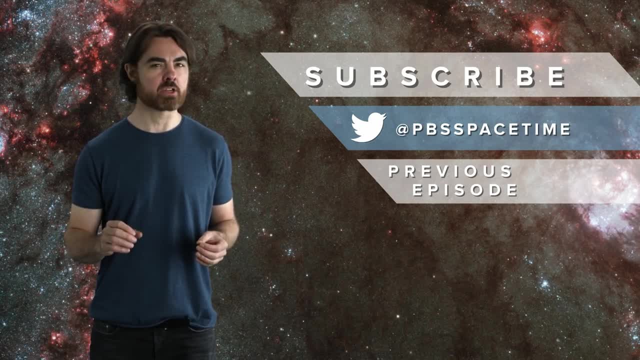 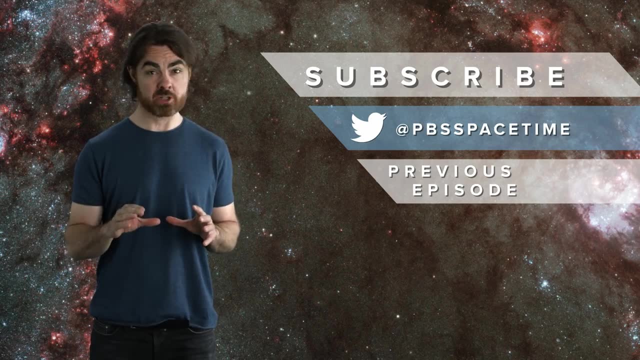 gravitationally lensed. Actually, yeah, The CMB is affected by weak lensing, so all of its blobs are very slightly distorted. This can change the power spectrum, so the distribution of the sizes of its blobs, which is really important for measuring.